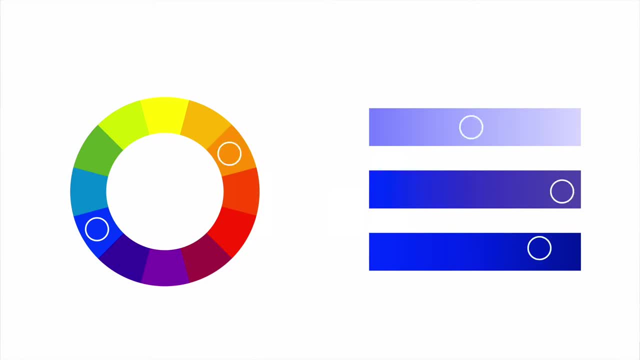 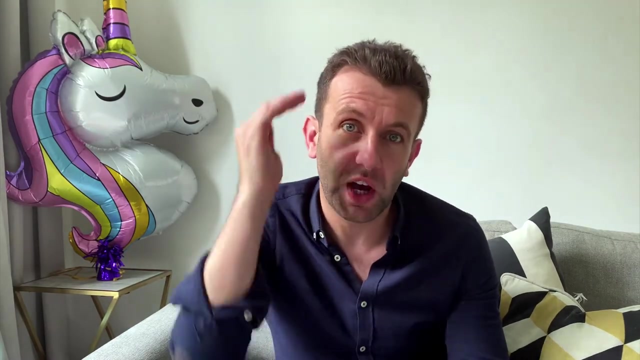 colour, but so is this, this and this. Artists and designers will call them hues, tints, tones and shades, but for this video, we're simply going to call them colours and gradients. Okay, now back to the colour palette. structures- Sequential. so when you have data values that go from low to high. 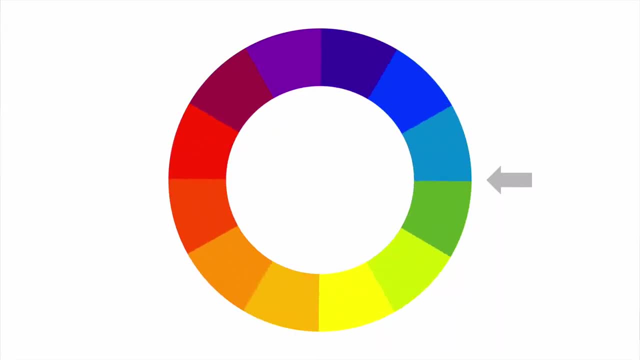 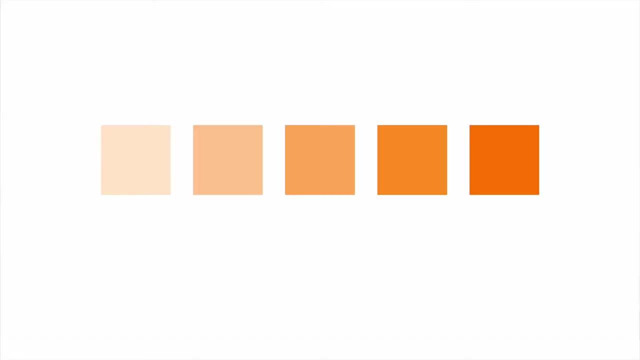 you need to stick with sequential colour palettes. Here you need to choose one colour or hue, but use a gradient of the colour. The one rule you have to follow with sequential palettes is that you need to make sure that the light colours represent the small numbers and that the darker colours. 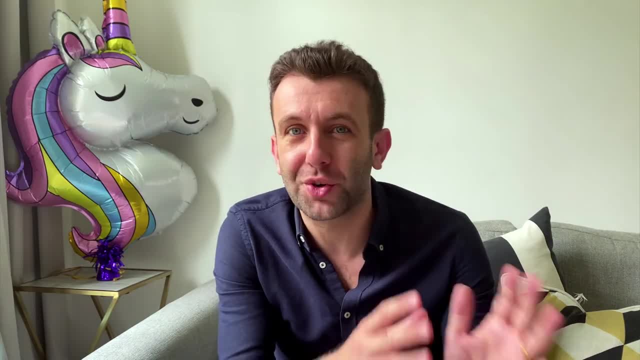 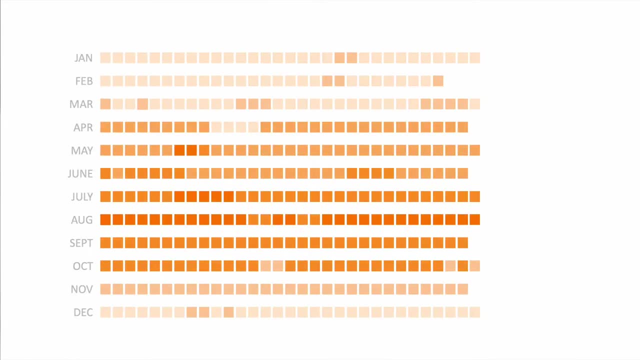 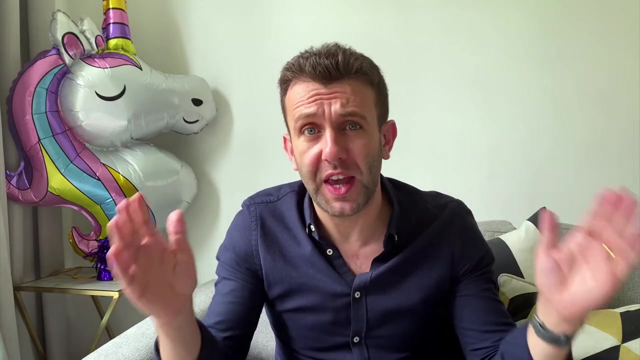 represent the larger numbers. Used right sequential colour palettes create numeric meaning, which means when we look at a data visualisation like this, we immediately get an idea of what the data is trying to show, without even showing any numbers, a key or a description. Not bad Divergent when you have data on a scale, but where the data separates into two. 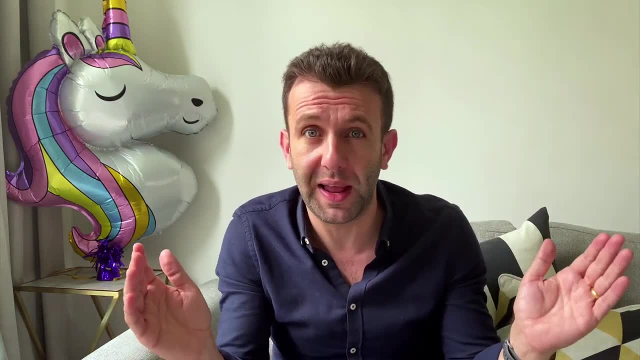 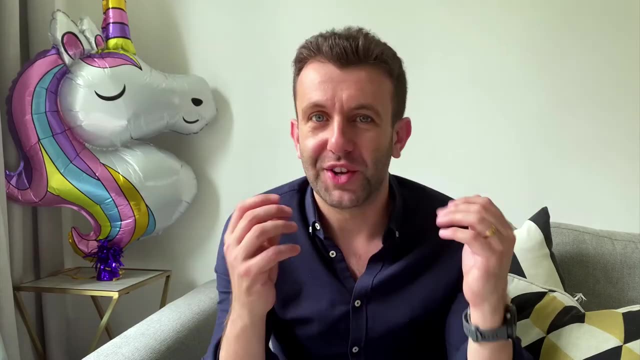 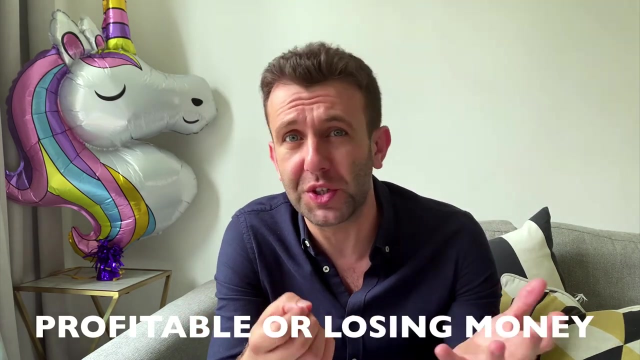 different sets. you want to use a divergent colour palette structure, So this is basically two different sequential colour palettes, often with a neutral midpoint. Divergent colour palettes are great for showing if people rated your company positive, If a customer is profitable or losing you money, or if temperatures are above freezing or below. 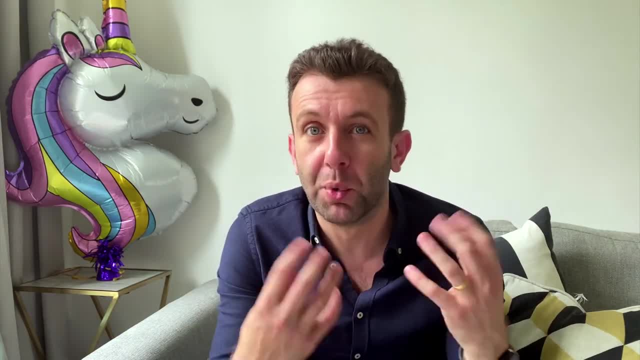 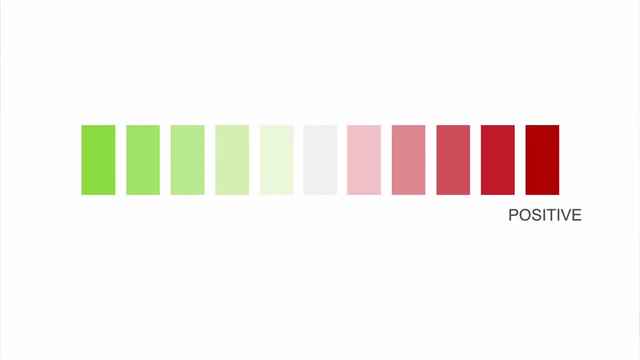 freezing things like that. Remember, though, that colours have meaning, and more so when you're using two colours in combination. You don't want to have blue symbolising hot and red symbolising cold, or red symbolising something positive and green negative. Spend a minute thinking about which two. 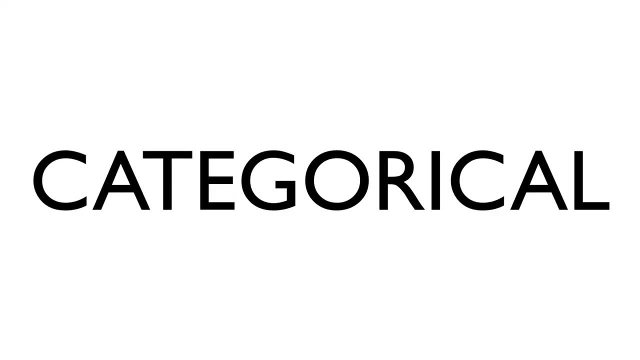 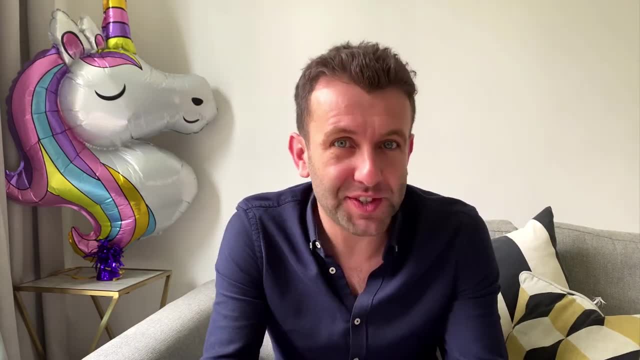 colours make the most sense for the data visualisation you want to create: Categorical, so sequential and divergent palettes. use colour to create numeric meaning, But when you're visualising data from different categories, your main goal is to show that this thing here is different to this thing here, So here you want to avoid using different. 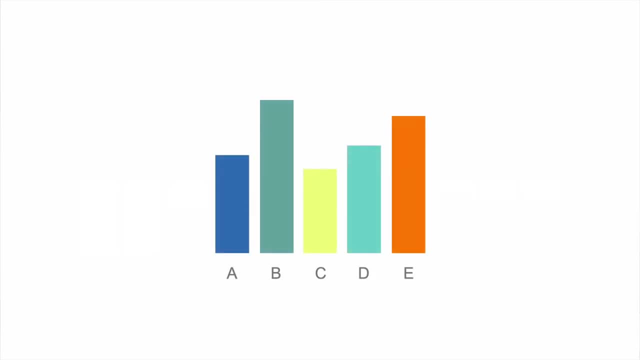 gradients of one or two colours, but instead use a range of distinctly different colours or hues. The main mistake people make with categorical colour palettes is using far too many colours. If you want it to be easy to understand, you really need to focus on having five categories.